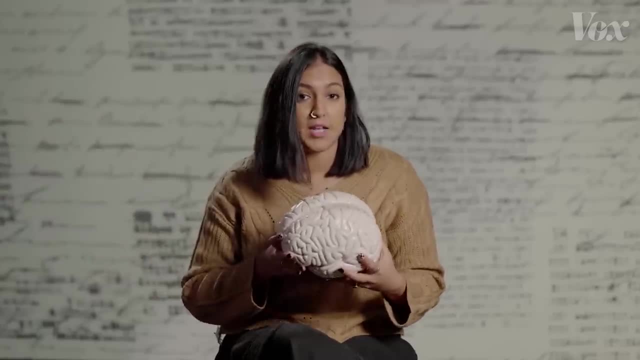 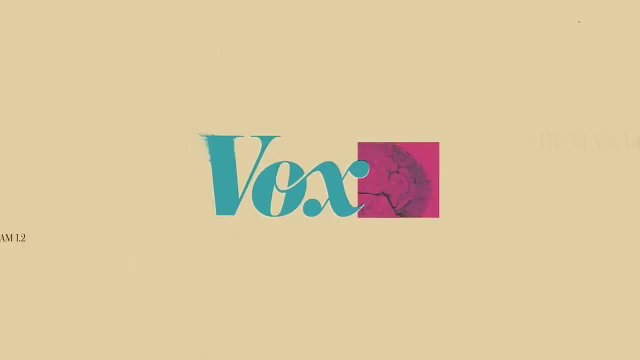 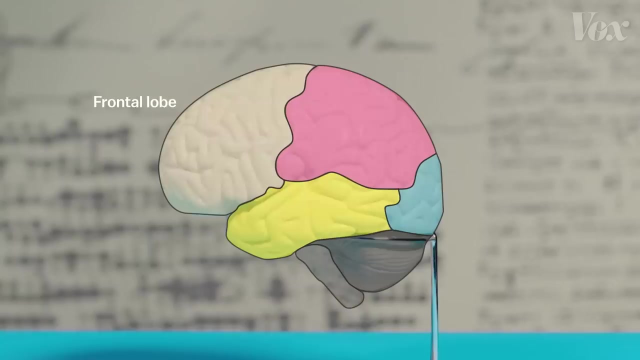 to here. The dyslexic brain is structured differently, in a way that can create specific challenges, but can also create specific advantages In terms of human evolution. the brain isn't naturally wired to read. There's not one specific region for reading, like there is for sleeping or engaging. our fear response. 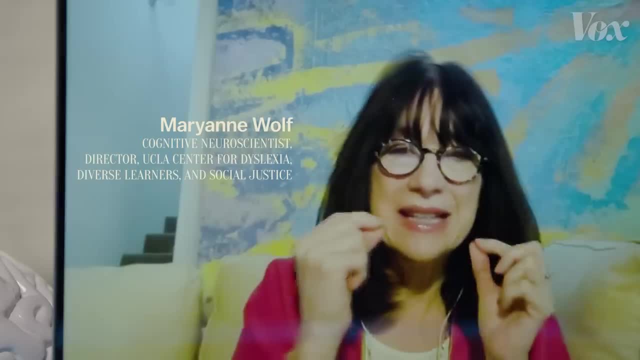 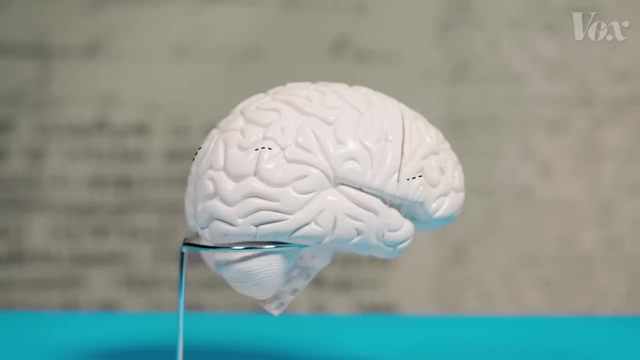 Reading. Reading is an issue. Reading is an issue. Reading is an issue. It is an invention that's only 6,000 years old. While there is so much we still don't understand about the human brain, over the past few decades, a clearer picture of how we read has emerged. 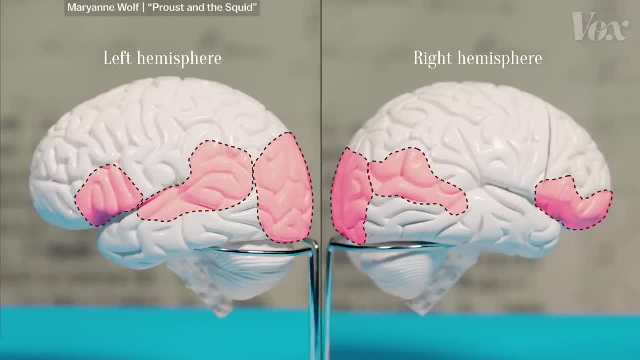 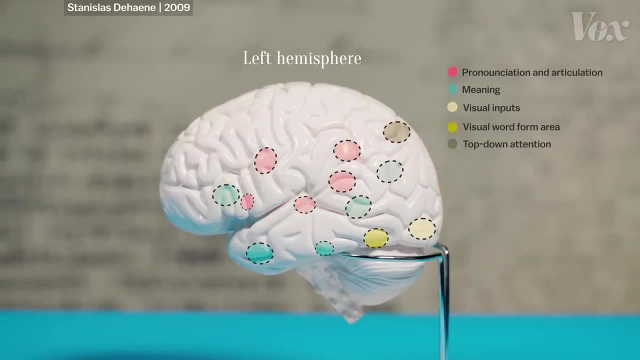 When we're young, we're activating both hemispheres of our brains, heavily, expending energy to learn how to read. But for fluent readers, the brain streamlines more activation to structures in the left hemisphere, like this region known as the visual word form area, which helps us recognize 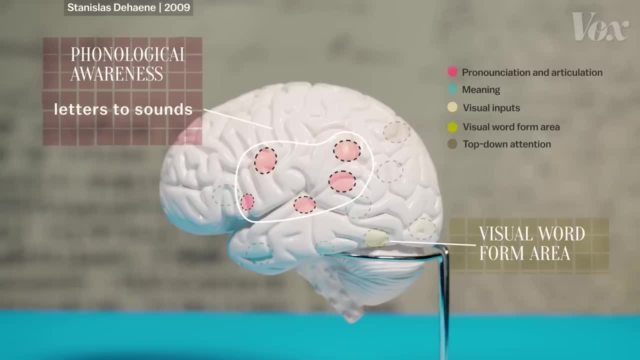 letters and words, And this region, key to mapping letters to sounds, called phonological awareness, For example, breaking up the word cat into the sounds ka, a and ta. And there's Broca's area, which, among other things, helps with comprehension. 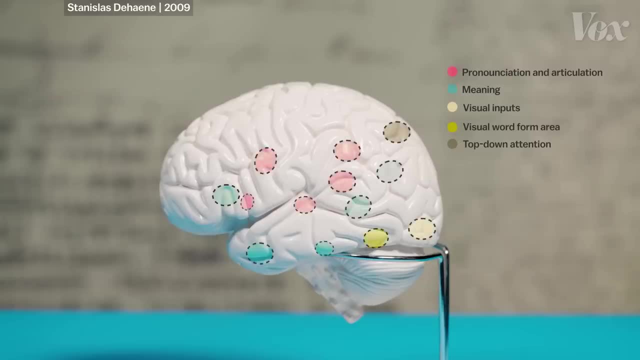 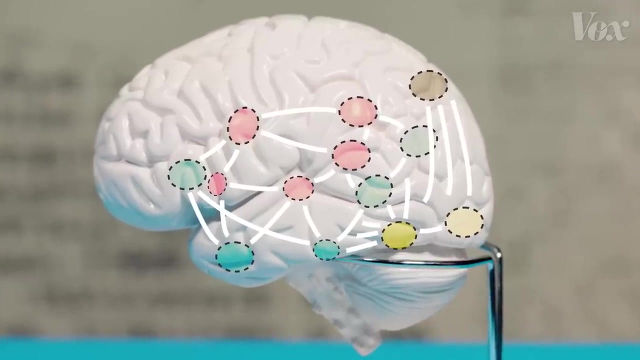 to understand what words actually mean. Activated areas link together with white matter. There are neural pathways that turn into a complicated highway network that allows fluent readers to process a word within milliseconds. BUT Even for the head-based brain, sometimes the larynx and the dyslexic brain, 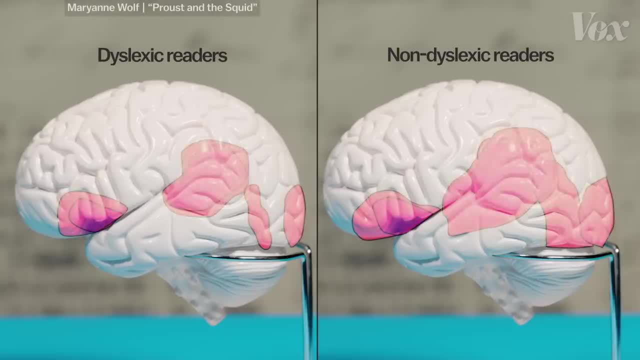 these highways and activated areas can look a lot different. Research using brain scans of dyslexic readers showed that there was less activation in these areas of the left hemisphere, suggesting there's often a pathway disruption in these systems that help map sounds to letters and decode words. 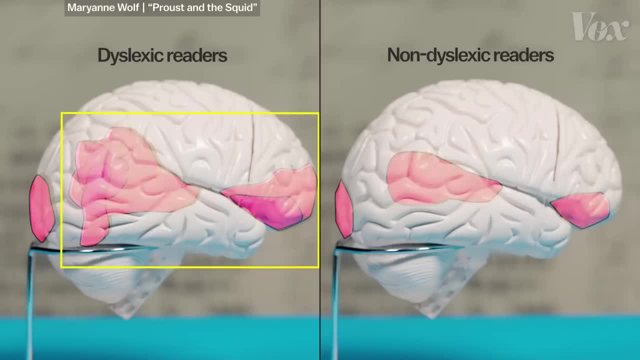 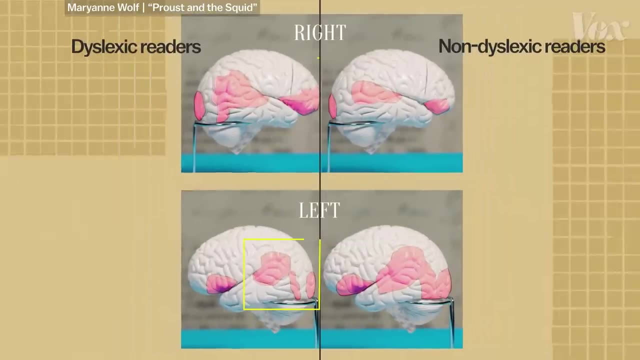 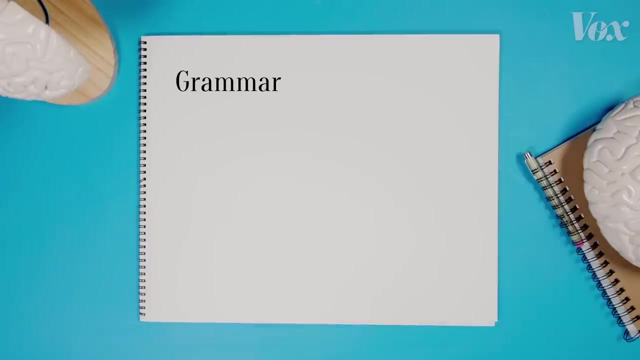 But people with dyslexia also consistently showed over-activation in the brain's right hemisphere when reading, And that makes it more laborious, may have trouble recognizing words and sounds. they're working even harder to compensate elsewhere. The pathway disruptions can also come with challenges in grammar, retrieving math facts. 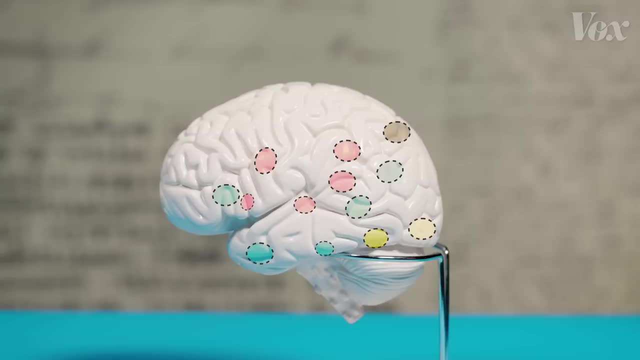 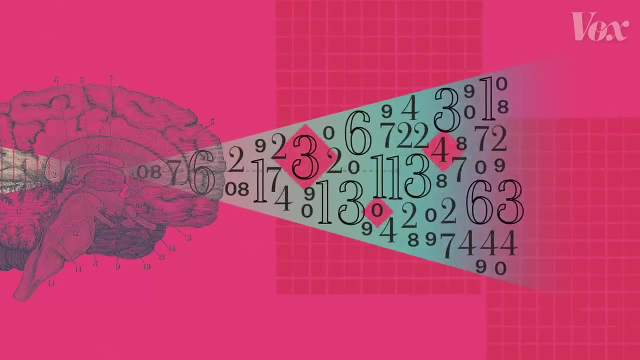 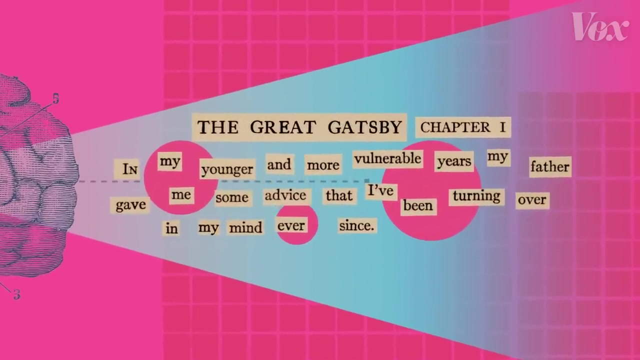 working memory, among other things too, Or often with dyslexia, neural pathways are not disrupted, but just slowed down. I'm sort of mildly dyslexic. My challenge is more with numbers Reading out loud in class. you're stricken with panic and then all the words start floating. 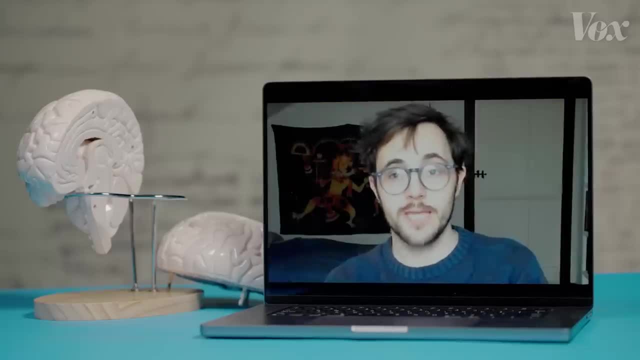 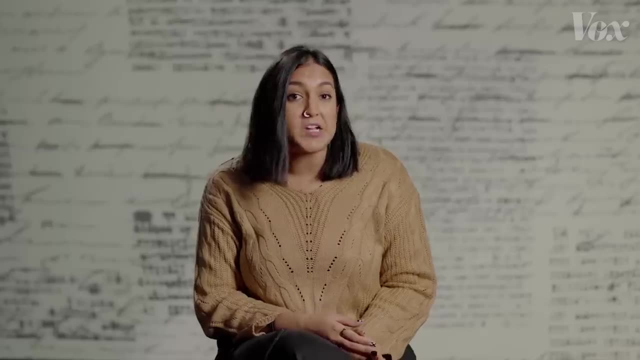 You just can't read the words. Everyone else would be on to doing the exercise and I'd be still trying to read the instructions. Exactly how people experience dyslexia varies greatly. It has no bearing on an individual's intelligence, but today it's commonly labeled a hereditary 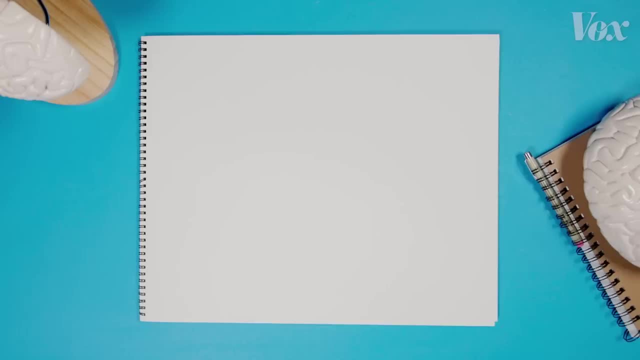 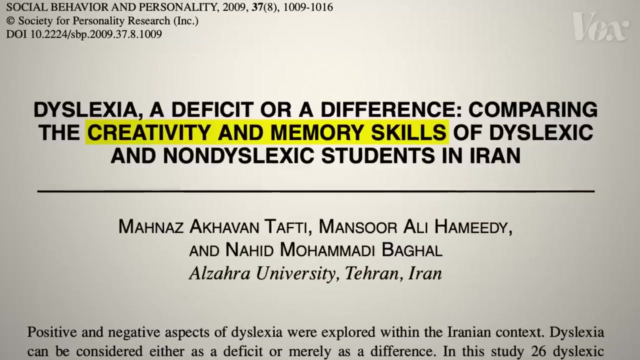 neurobiological learning disability Research has found explicit support, and instruction in areas like phonology, syntax and spelling can lead to success for dyslexic learners. But the reading brain Is only part of the picture. Years of research has started corroborating the idea that dyslexic people are prone to 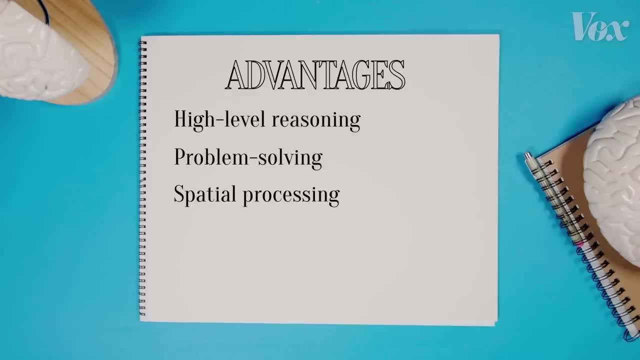 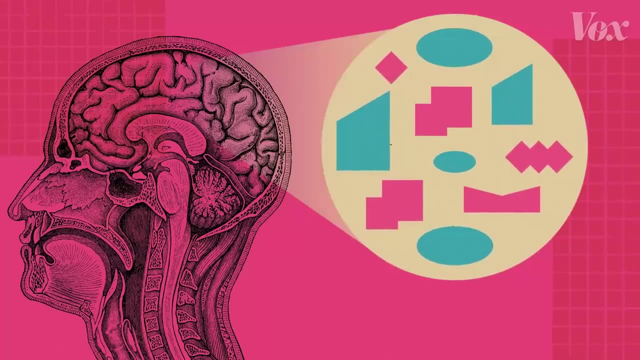 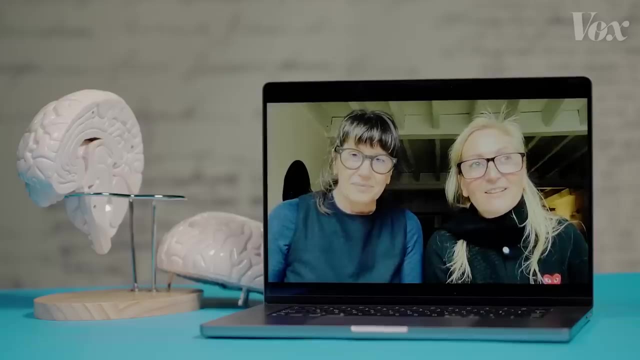 advantages, including high-level reasoning, problem solving, spatial processing, episodic memory and creativity, Because I have the full picture in my head, sometimes I can make association between things that they don't appear to be relevant. We shake it up a bit if we kind of get people to think: you know, oh, I didn't think of. 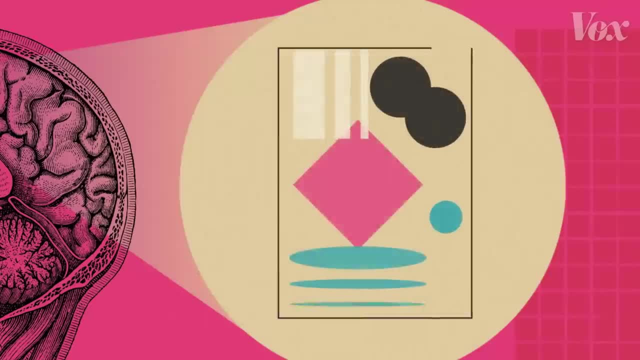 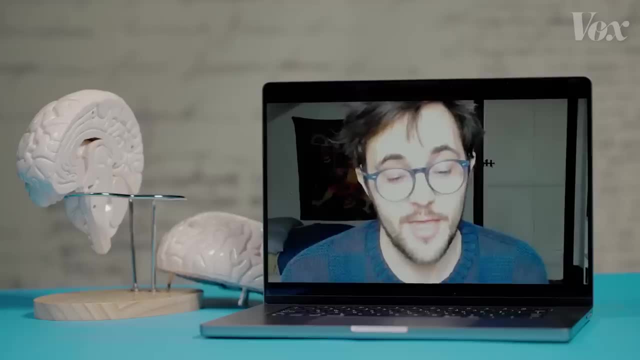 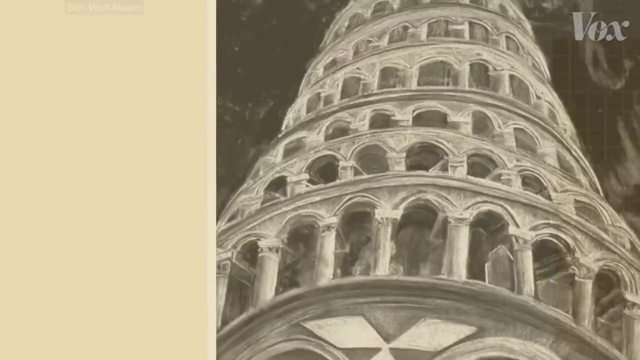 that Sometimes we recall images. I'll meet somebody and I will stop them on the street and be like we know each other, and they will have no idea. I'm going to show you what a dyslexic high schooler did. I was floored, gobsmacked, because he was drawing from memory upside down. 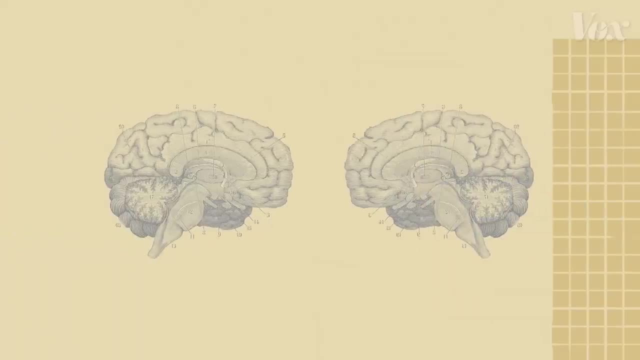 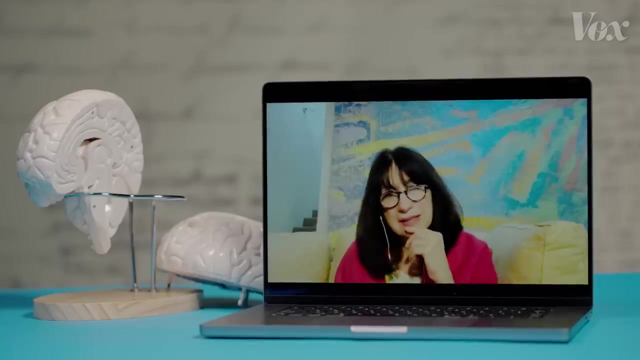 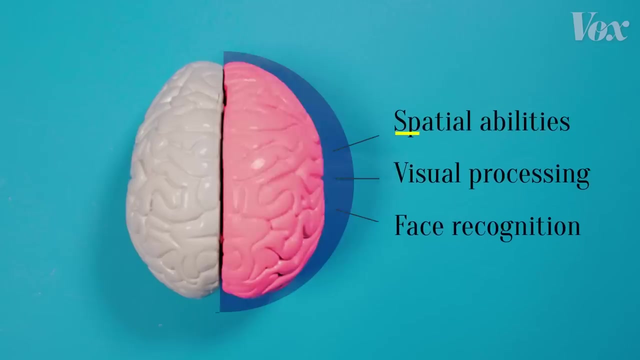 There are specific areas of strength in the right hemisphere that seem very much to be at play. We can't see with individuals with dyslexia. While most functions do use both hemispheres of our brains, the right hemisphere is typically associated with skills like spatial abilities and visual imagery. 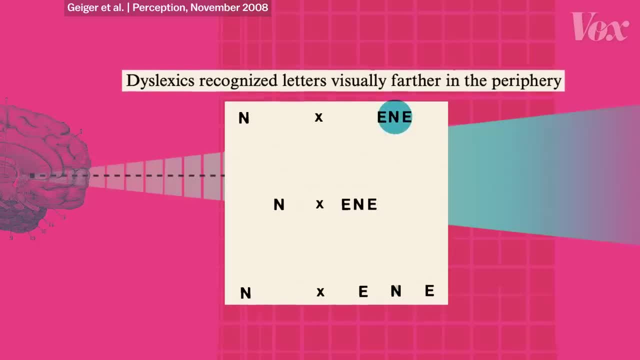 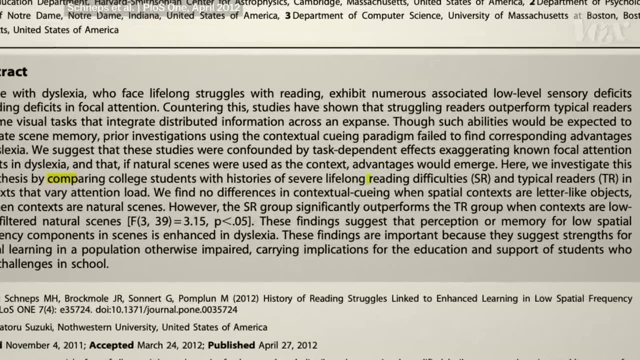 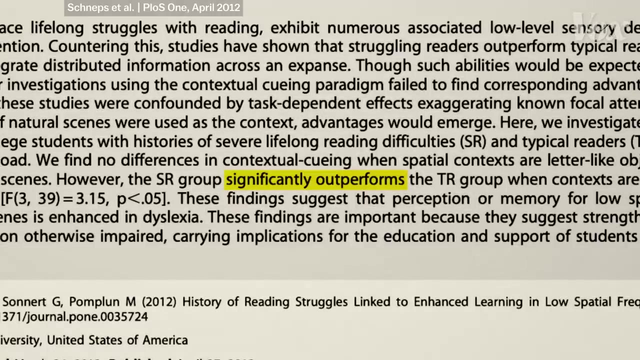 In a study similar to the one with impossible figures, dyslexic people were better able to identify letters in their periphery than other readers. Another study compared the abilities of college students with and without dyslexia to memorize blurred images. Students with dyslexia significantly outperformed.